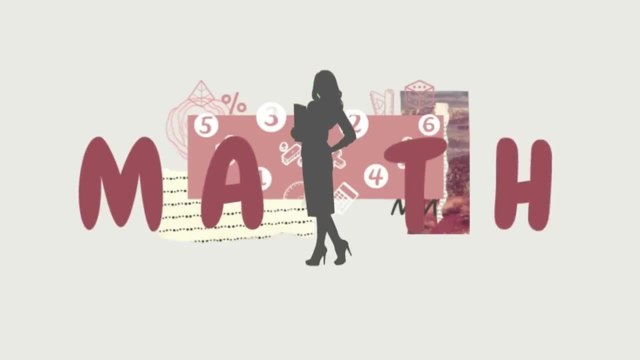 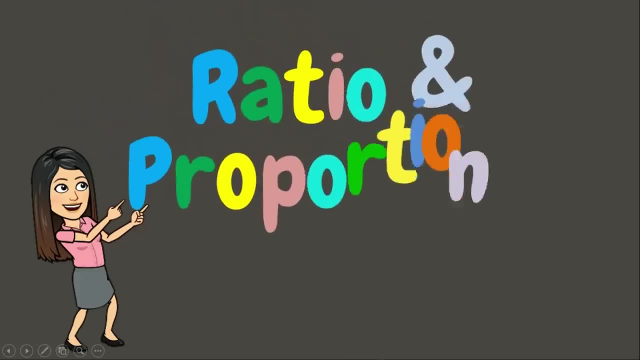 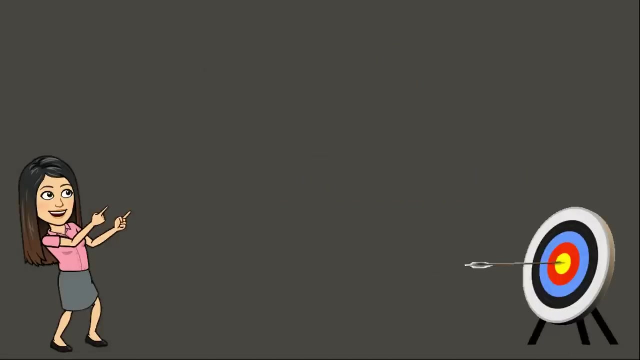 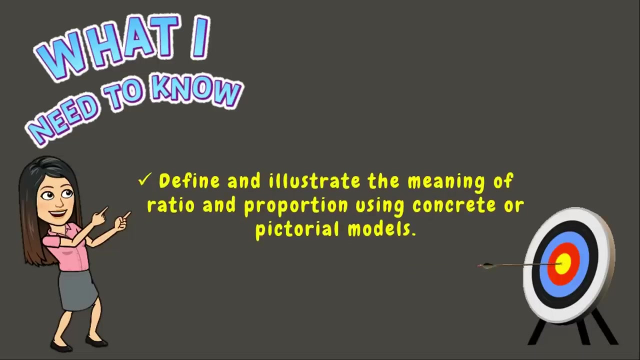 Ratio and Proportion. Great day students. Welcome back to my classroom For today's lesson. you will learn how to define and illustrate the meaning of ratio and proportion using concrete or pictorial models. Let's begin. Let's have our first example. 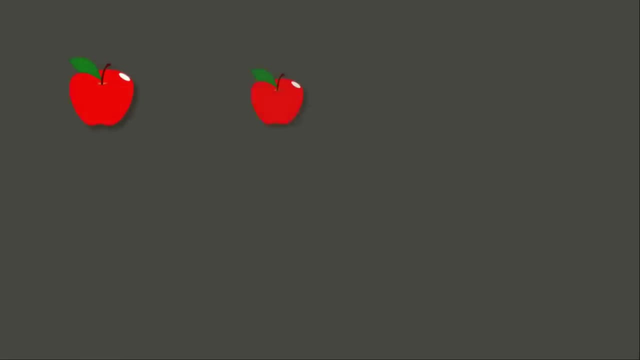 I bought three apples and six mangoes for my milkshake. Now the question is: what is the ratio of apples to mangoes? Hmm, but wait, what is ratio? Well, ratio is the ratio of apples to mangoes. It's a way of comparing two or more quantities. 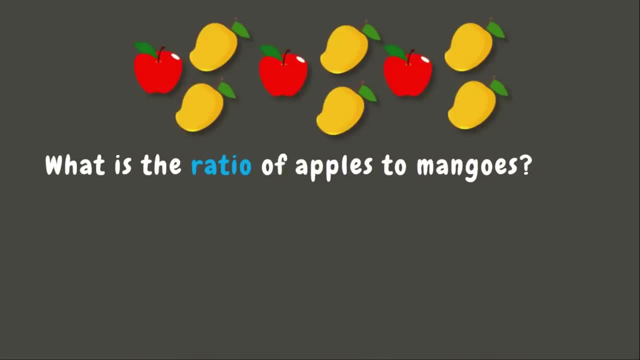 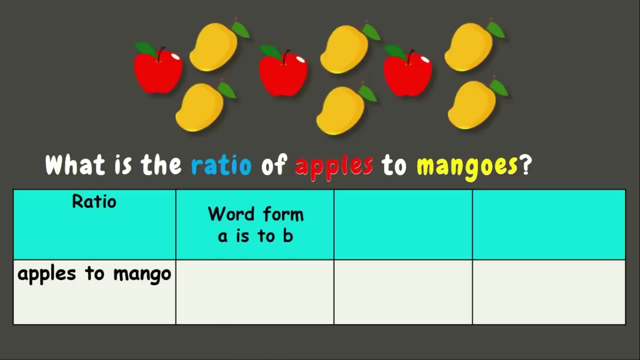 Here we are asked to get the ratio or compare the quantity or number of apples to mangoes. We have three ways in writing a ratio. The first one is the word form, which is A is to B. Here we are going to count first the first item, which is the apples. 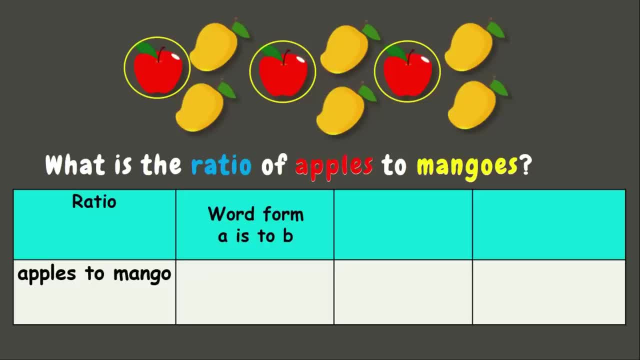 We have three apples. Let's write three. Three is two. The second item is to mango. We have six mangoes. That makes three is to six. Wonderful, Now for our second way in writing a ratio. we have the colon form. 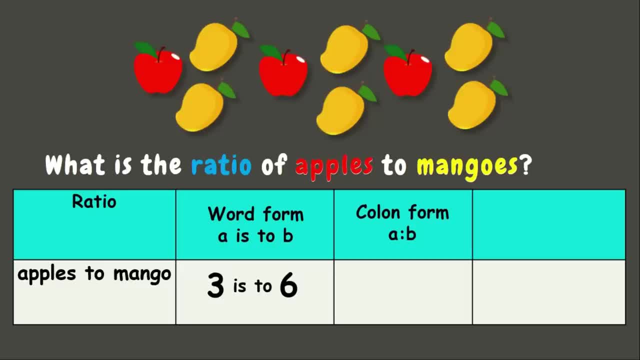 Here, instead of writing the word is to, we are going to replace it by the colon symbol. That makes three colon six, But still read as three is to six. Finally, our last way of writing the ratio is the fraction form, where the first quantity serves as the numerator while the second quantity serves as the denominator. 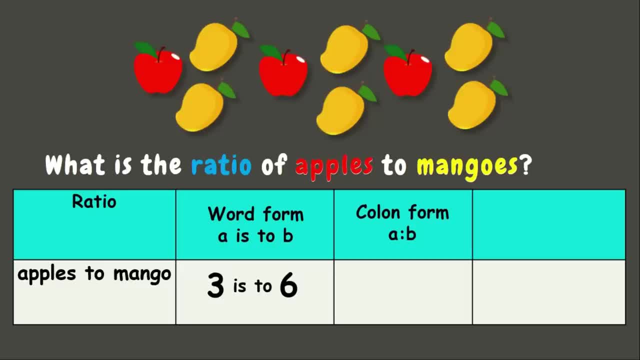 Here, instead of writing the word is to, we are going to replace it by the colon symbol. That makes three colon six, But still read as three is to six. Finally, our last way of writing the ratio is the fraction form, where the first quantity serves as the numerator while the second quantity serves as the denominator. 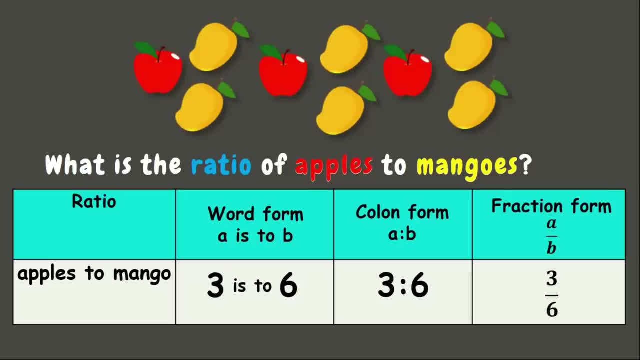 which makes three, Three over six. This means that for every three apples, we have six mangoes. Remember, ratio is a comparison of two or more quantities, But we can only use the fraction form when we are only comparing two quantities. Wonderful. 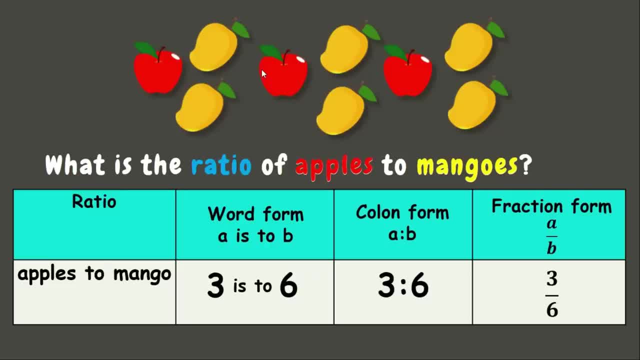 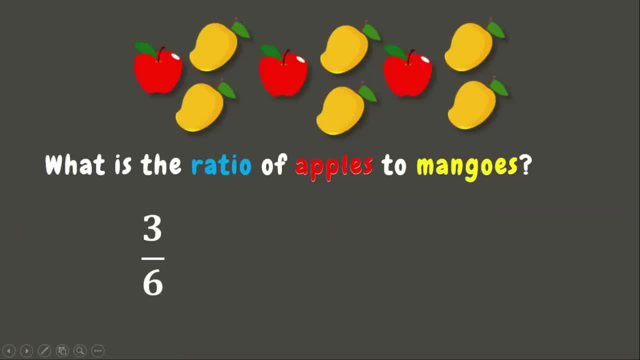 Now, like fraction, ratios can be simplified into Lobby's Term as well. Let me give you an example. We have three over six, or three is to six. We can simplify the ratio into Lobby's Term, like how we simplify a fraction, by dividing both quantities by its greatest common factor. 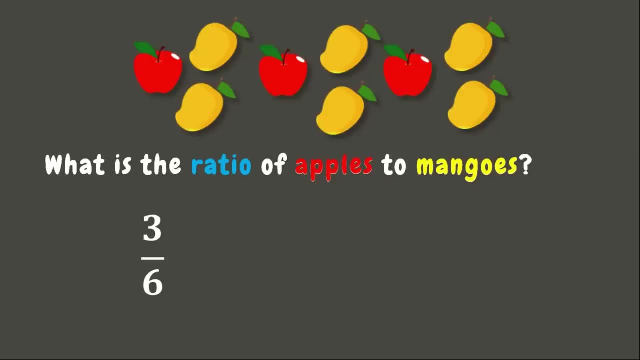 Here the greatest common factor of three and six is very good three. Now let's divide three by three and six by three. That gives us one is to two. This means that for every one apple we have two mangoes. 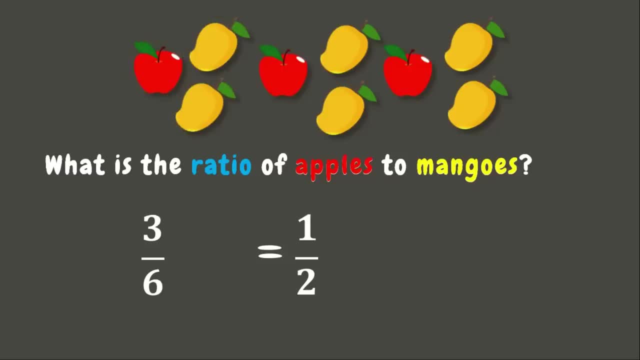 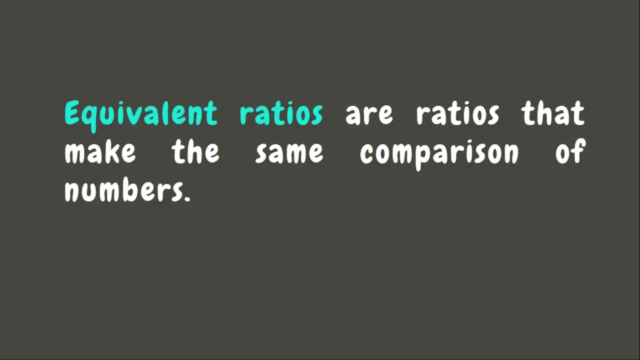 This also means that three, six is equivalent to one half, or three is to six is equivalent to one is to two. This is an example of equivalent ratio. Equivalent ratios are ratios that make the same comparison of numbers. Now how do we get the equivalent of the ratios? 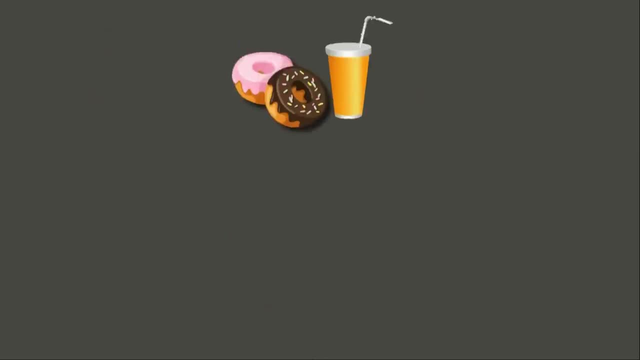 Let me give you an example. I have here two donuts and one drink. It means that the ratio of the drink to donuts is one is to two. We can also write the ratio one is to two into its fraction form one half. 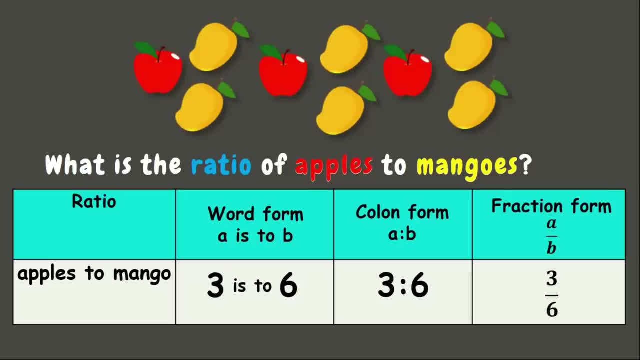 which makes three, Three over six. This means that for every three apples, we have six mangoes. Remember, ratio is a comparison of two or more quantities, But we can only use the fraction form when we are only comparing two quantities. Wonderful. 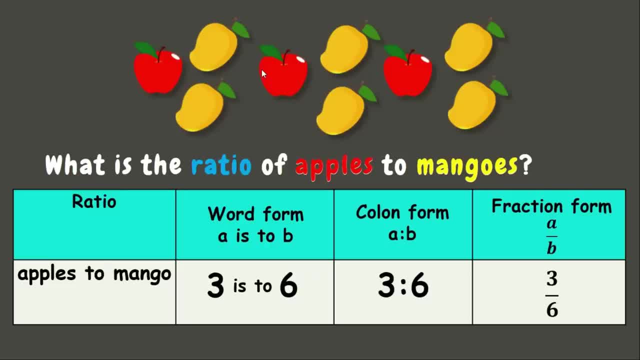 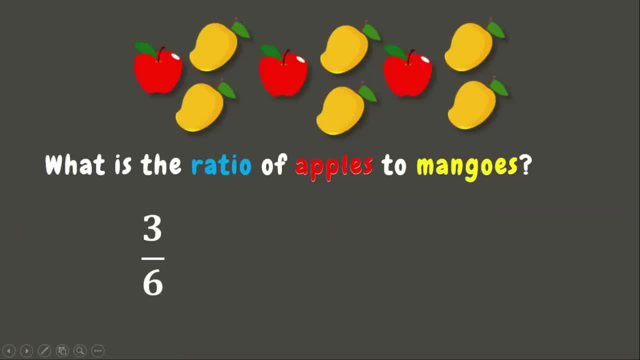 Now, like fraction, ratios can be simplified into Lobby's Term as well. Let me give you an example. We have three over six, or three is to six. We can simplify the ratio into Lobby's Term, like how we simplify a fraction, by dividing both quantities by its greatest common factor. 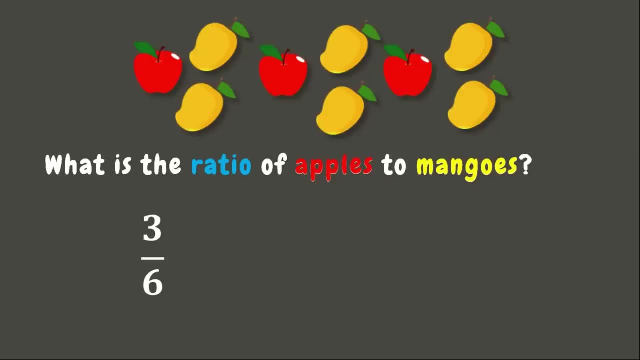 Here the greatest common factor of three and six is very good three. Now let's divide three by three and six by three. That gives us one is to two. This means that for every one apple we have two mangoes. 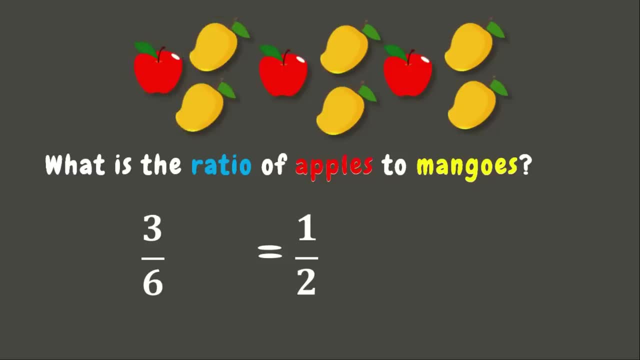 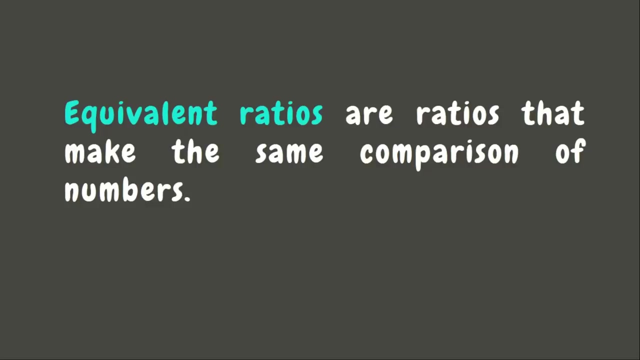 This also means that three, six is equivalent to one half, or three is to six is equivalent to one is to two. This is an example of equivalent ratio. Equivalent ratios are ratios that make the same comparison of numbers. Now how do we get the equivalent of the ratios? 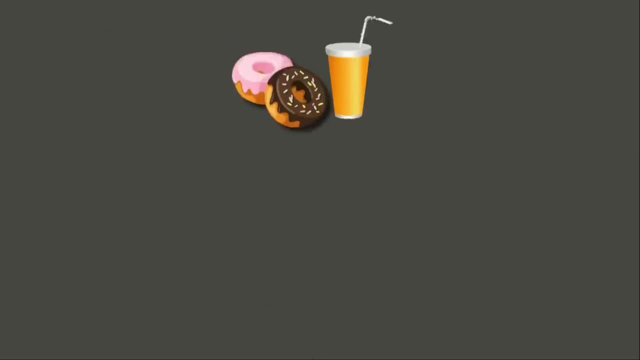 Let me give you an example. I have here two donuts and one drink. It means that the ratio of the drink to donuts is one is to two. We can also write the ratio one is to two into its fraction form one half. 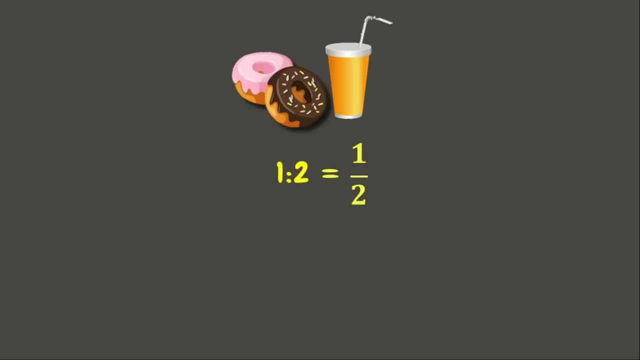 Now to get the equivalent of the ratios, we are just going to simply multiply both quantities by any number. Let's say, for example: let's multiply one half by two: One times two is two. Two times two is four. This means that one half or one is to two is equivalent to two is to four. 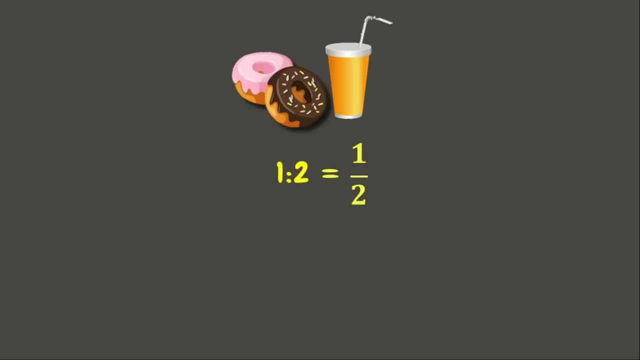 Now to get the equivalent of the ratios, we are just going to simply multiply both quantities by any number. Let's say, for example: let's multiply one half by two: One times two is two. Two times two is four. This means that one half or one is to two is equivalent to two is to four. 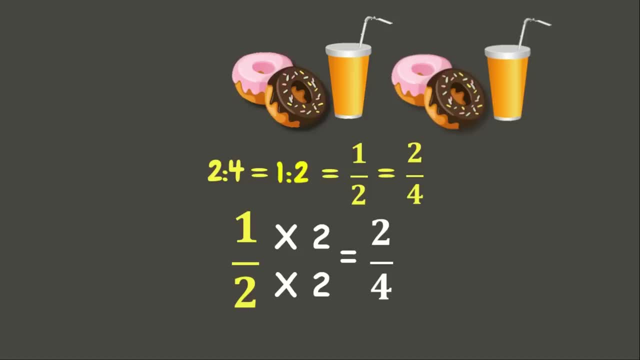 Now let's try to multiply this by three. We get three over six, or three is to six. This also means that one is to two and two is to four. Four is equivalent to three is to six. Wonderful, Now we can also get the equivalent of a ratio by dividing both quantities by its factor. 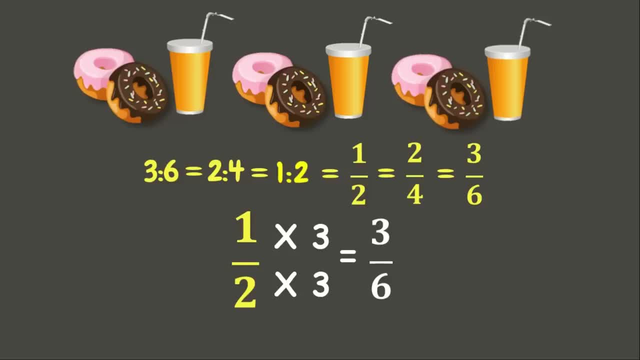 We know that the factor of three and six is three. Three divided by three is one, while six divided by three is two. This means that three is to six is equivalent to one is to two. Three divided by three is equivalent to one, is to two. 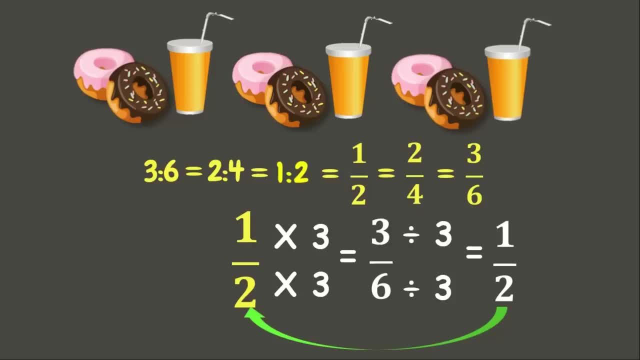 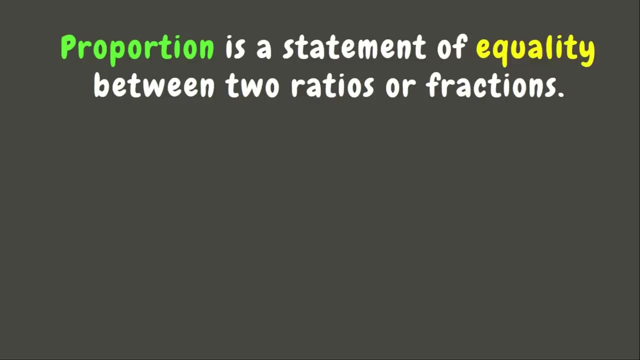 Very good. Again, these are what we call equivalent ratios, But this also shows proportion. Do you know what a proportion is? Proportion is a statement of equality between two ratios or fractions. Let me give you an example: One is to three is equivalent, or proportion to three is to nine. 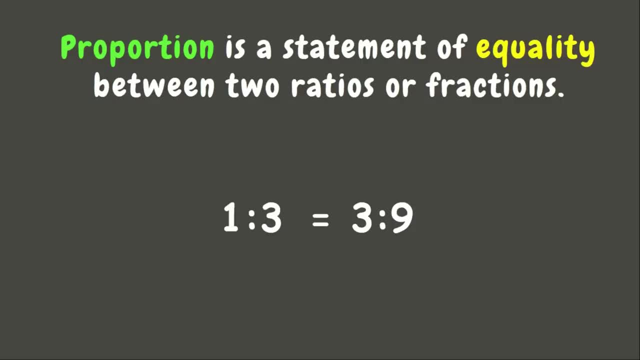 There are two parts in a proportion. The numbers we find inside are what we call means, while the number outside are extremes. We will know if the ratios are proportioned to each other if the product of the means and the extremes are equal. Now let's try. 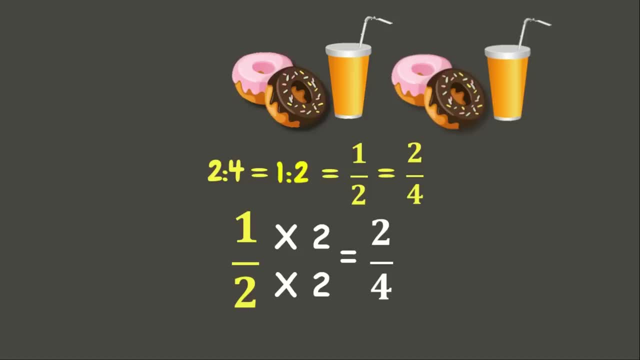 Now let's try to multiply this by three. We get three over six, or three is to six. This also means that one is to two and two is to four is equivalent to three is to six. Wonderful, Now we can also get the equivalent of a ratio by dividing both quantities by its factor. 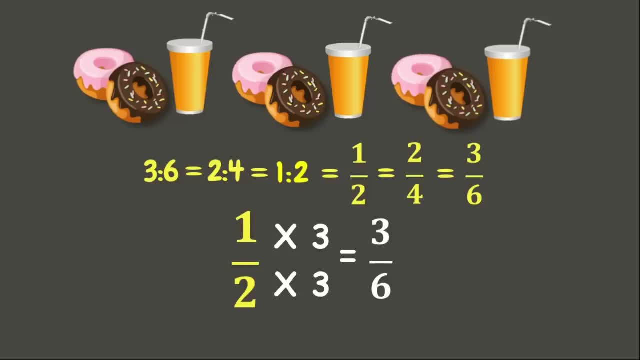 We know that the factor of three and six is three. Three divided by three is one, while six divided by three is two. This means that three is to six is equivalent to one is to two. Very good, Again, these are what we call equivalent ratios. 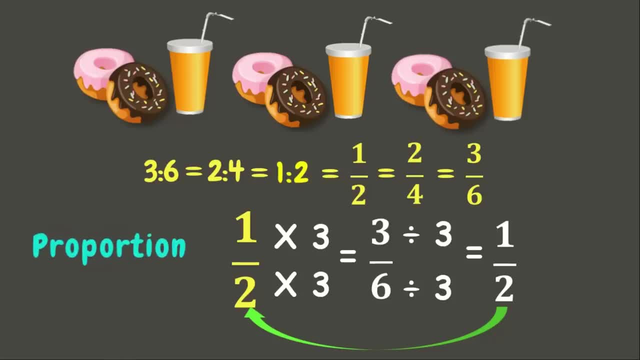 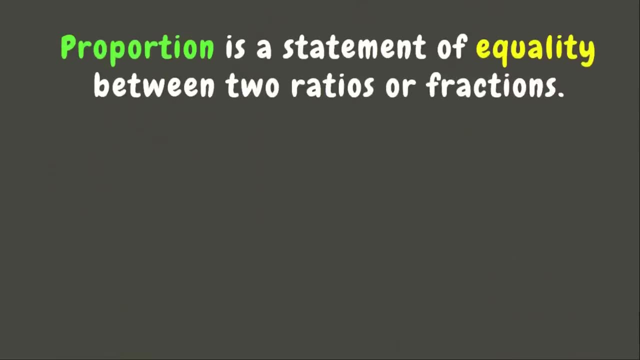 But this also shows proportion. Do you know what a proportion is? Proportion is a statement of equality between two ratios or fractions. Let me give you an example. One is to three, Two is equivalent, or proportion to three is to nine. There are two parts in a proportion. 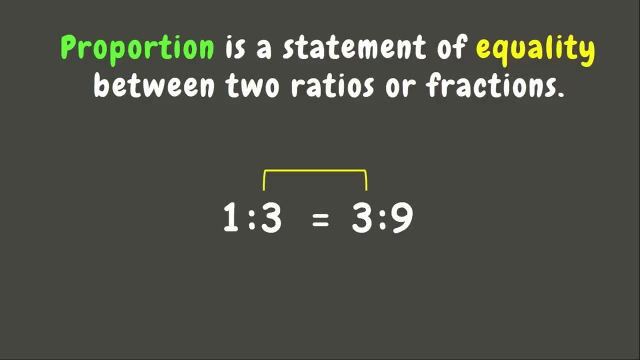 The numbers we find inside are what we call means, While the number outside are extremes. We will know if the ratios are proportion to each other if the product of the means and the extremes are equal. Now, let's try. Let's multiply the means. 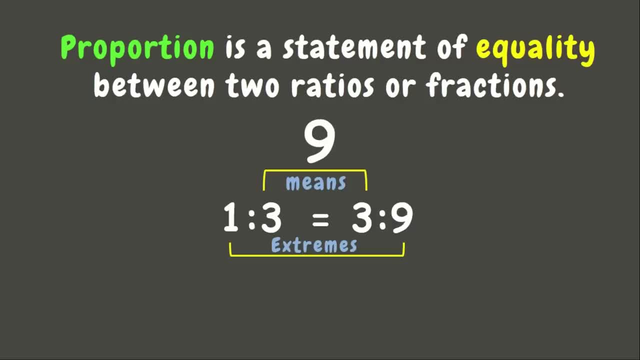 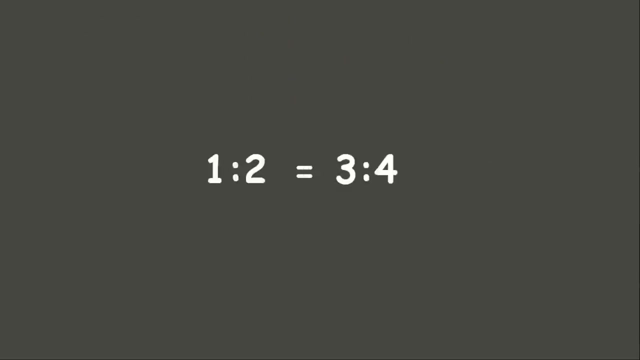 Three times three is nine. Now let's multiply the extremes Nine times one is nine. Here we can see that their products are both nine. This means that they are proportion. Let's have another example. I have here proportion. one is to two equals three is to four. 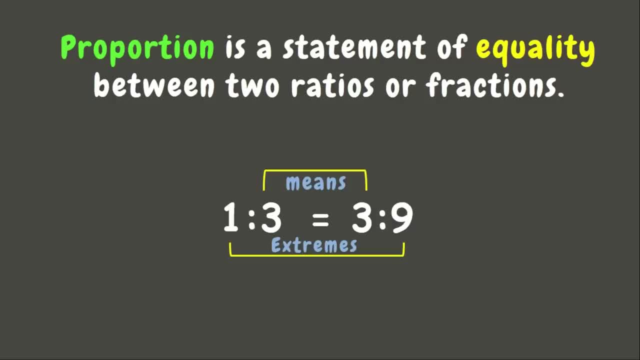 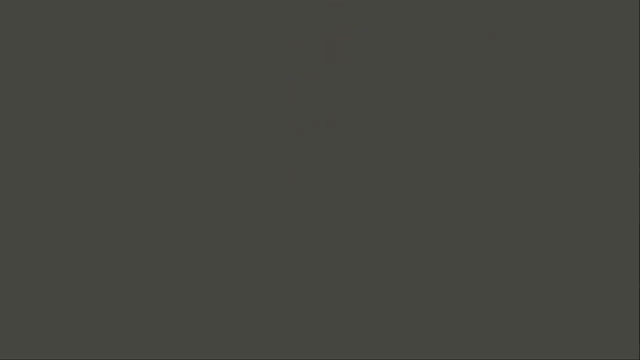 Let's multiply the means Three times three is nine. Now let's multiply the extremes Nine times one is nine. Here we can see that their products are both nine. This means that they are proportioned. Let's have another example. I have here proportion: one is to two equals three is to four. 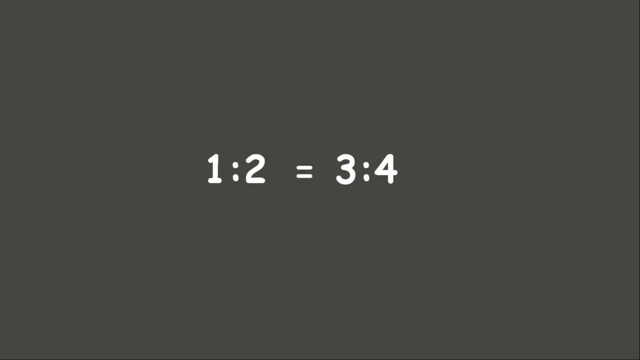 Now let's see if they are proportioned to each other. Let's multiply the means: Three times two is six. Now let's multiply the extremes: One times four is four. Now are they equal? No, Six and four are not equal to each other. 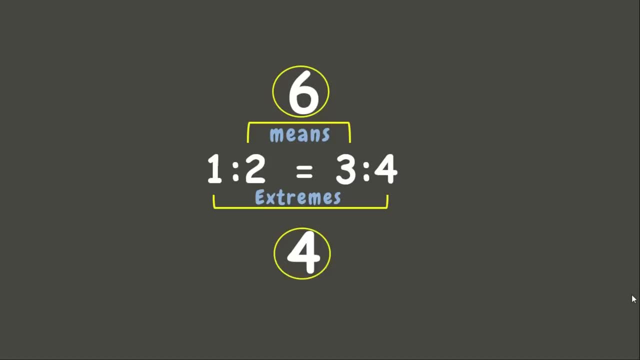 This means that the ratio one is to two and three is to four are not proportioned to each other. Now let's have another example. Let's try to find out if these fraction forms are equivalent or proportioned to each other. To determine if they are proportioned: 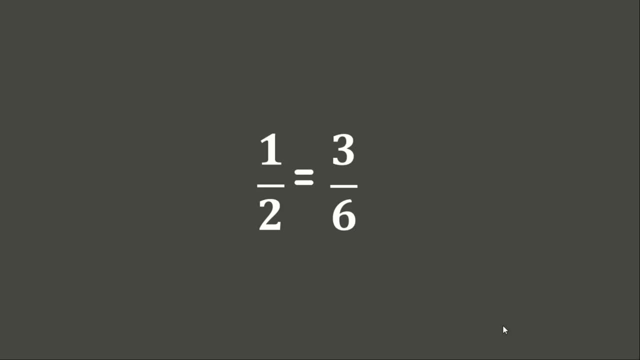 let's use the cross multiplication method. Six times one is six, While two times three is six. Since the products are both six, that means they are proportioned to each other. Let's have one more example. How about these ratios and fraction forms? 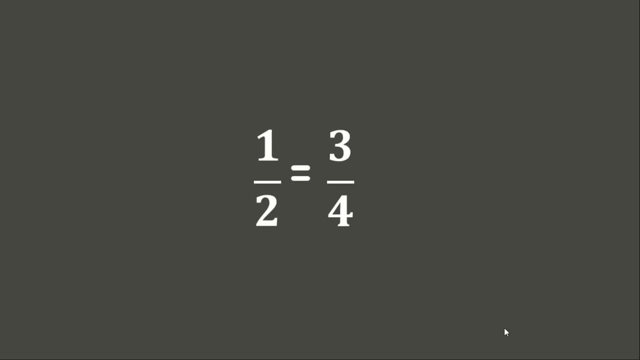 One is to two equals three is to four. Let's use the cross multiplication method: Four times one is four, While two times three is six, Since the products are not the same and four is not equal to six. this means that these two ratios 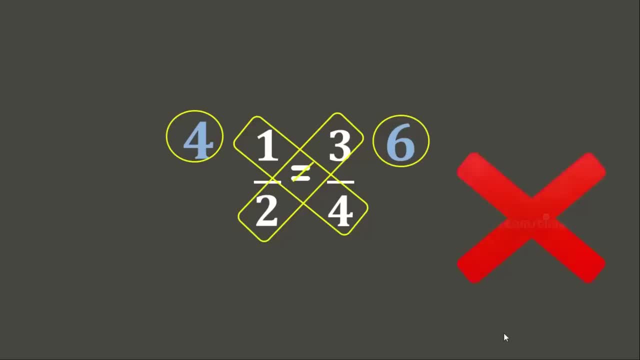 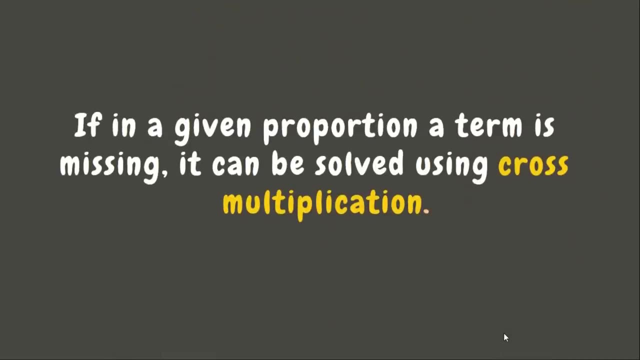 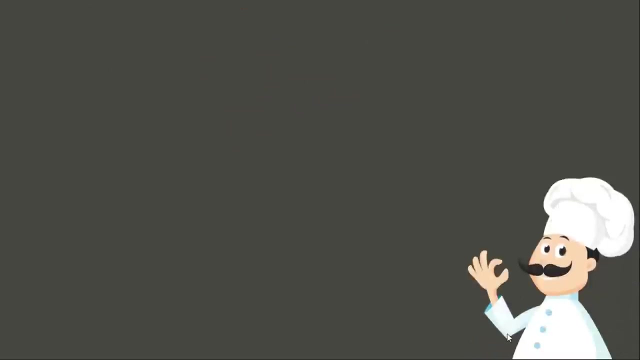 are not proportioned to each other. Great job. Now, if, in a given proportion, a term is missing, it can be solved using cross multiplication. Let me show you an example. Let's say a baker can bake a cake using two cups of flour. 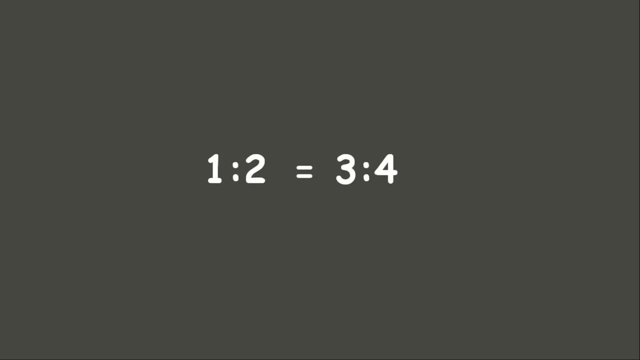 Now let's see if they are proportion to each other. Let's multiply the means: Three times two is six. Now let's multiply the extremes: One times four is four. Now are they equal? No, Six and four are not equal to each other. 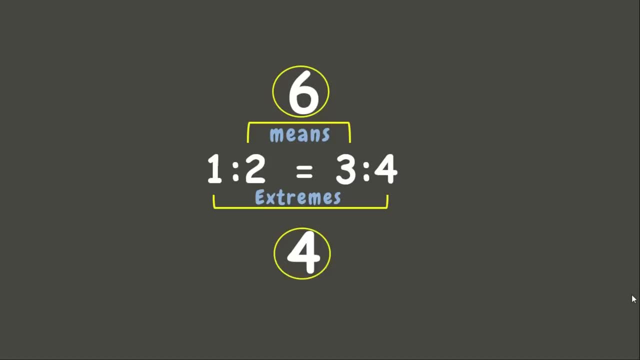 This means that the ratio one is to two and three is to four are not proportion to each other. Now let's have another example. Let's try to find out if these fraction forms are equivalent or proportion to each other. To determine if they are proportion. 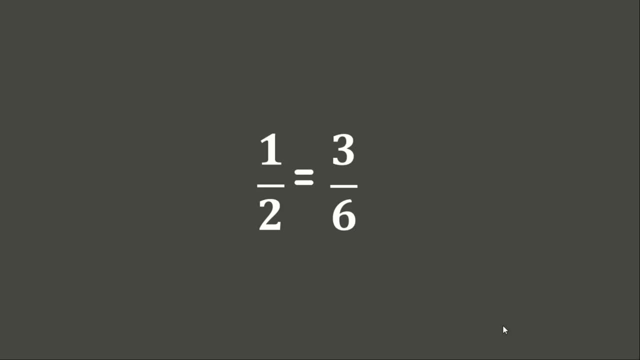 Let's use the cross multiplication method. Six times one is six, While two times three is six. Since the products are both six, That means they are proportion to each other. Let's have one more example. How about these ratios and fraction forms? 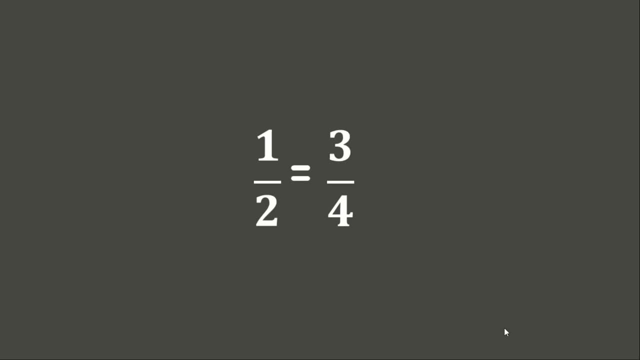 One is to two equals three is to four. Let's use the cross multiplication method: Four times one is four, While two times three is six, Since the products are not the same And four is not equal to six. This means that these two ratios are not proportion to each other. 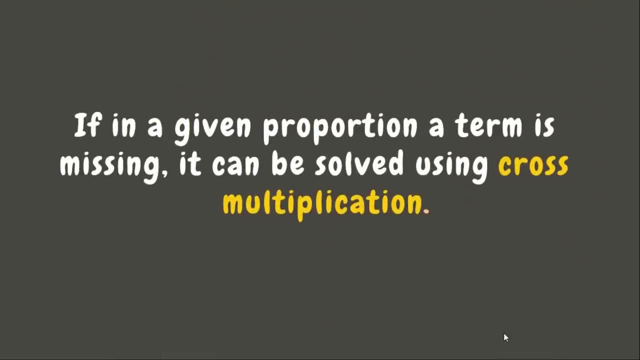 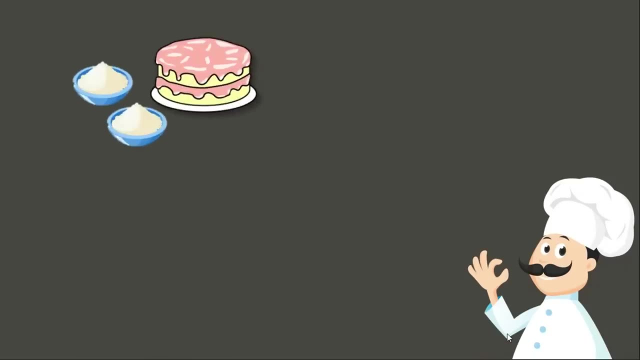 Great job. Now, if, in a given proportion, A term is missing, It can be solved using cross multiplication. Let me show you an example. Let's say a baker can bake a cake Using two cups of flour. This gives us the ratio of the cup of flour to the cake. 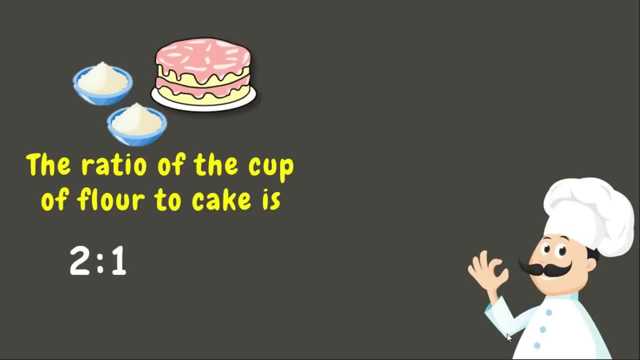 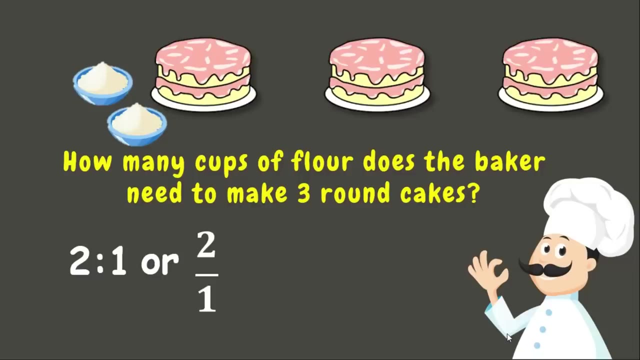 Which is two, is to one, or two over one. Now the baker needs to make three cakes. The question is: How many cups of flour does the baker need to make three round cakes? The first thing that we need to know are the quantities given. 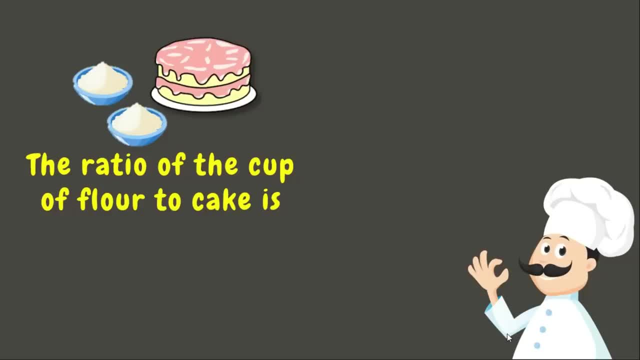 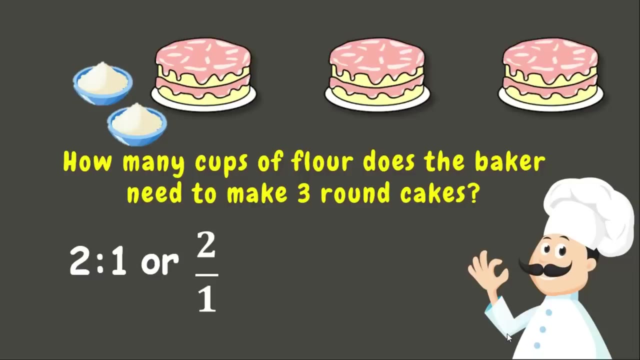 This gives us the ratio of the cup of flour to the cake, which is two is to one, or two over one. Now the baker needs to make three cakes. The question is: how many cups of flour does the baker need to make three round cakes? 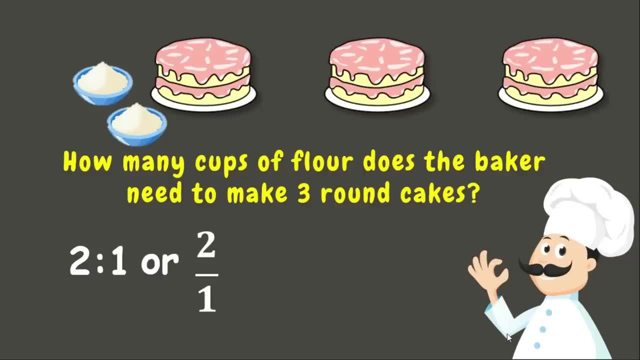 The first thing that we need to know are the quantities given. We have the number of cups of flour, which is two, and the number of cake that we can make, which is one. We know that for every two cups of flour, we can make one cake. 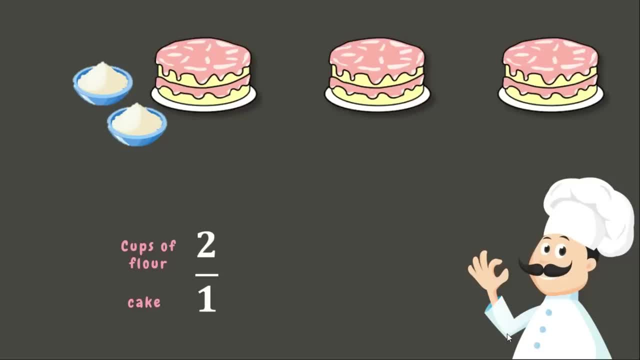 Now let's set up a proportion. The problem is: what if we make three cakes? How many cups of flour should we have? Since we do not know yet, let's write n Now to find the missing term, which is n. 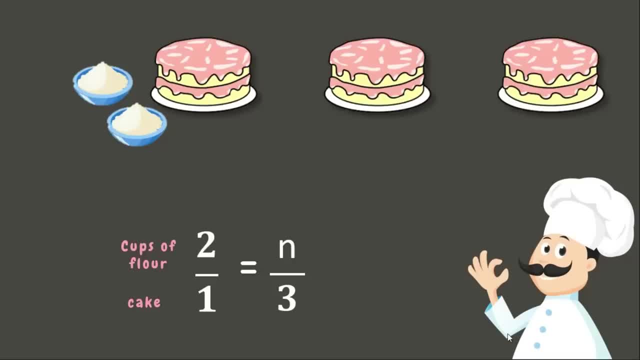 let's use the cross multiplication: Three times two is six, While one times n is one n, but we are only going to write one. The next step is to divide the products. Six divided by one is six, Great job. This means that we need six cups of flour. 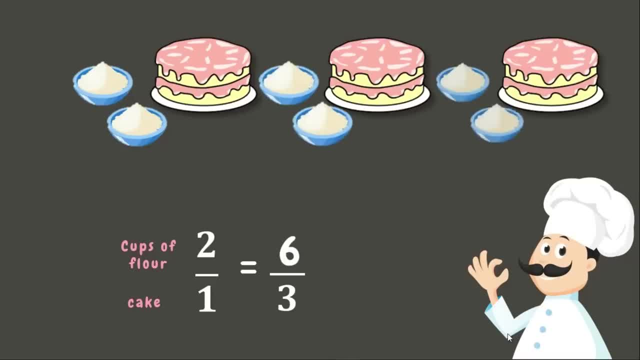 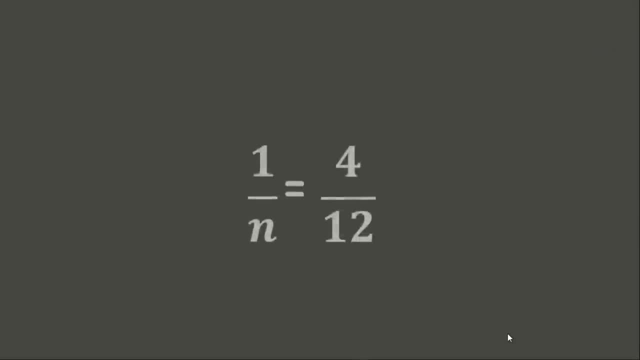 to make three round cakes- Wonderful. Let's have another example. Let's say we have this proportion. Let's find the missing term. Again, we will use cross multiplication method. Twelve times one is twelve, n times four is four, n. 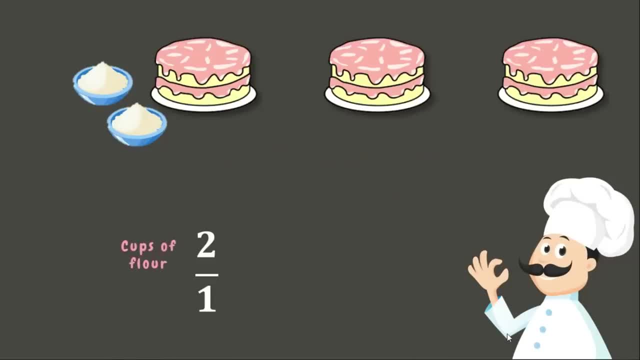 We have the number of cups of flour, Which is two, And the number of cake that we can make, Which is one. We know that for every two cups of flour, We can make one cake. Now, let's set up A proportion. 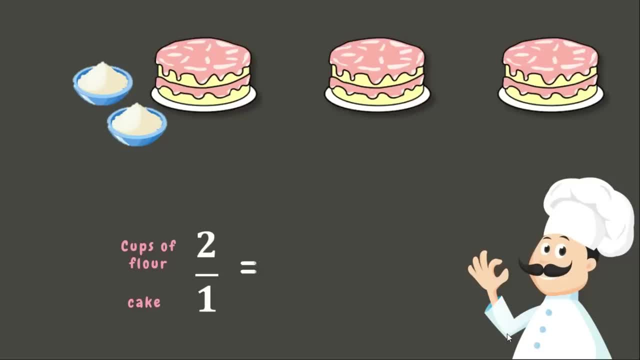 The problem is: What if we make three cakes? How many cups of flour should we have? Since we do not know yet, Let's write n Now to find the missing term, Which is n. Let's use the cross multiplication: Three times two is six. 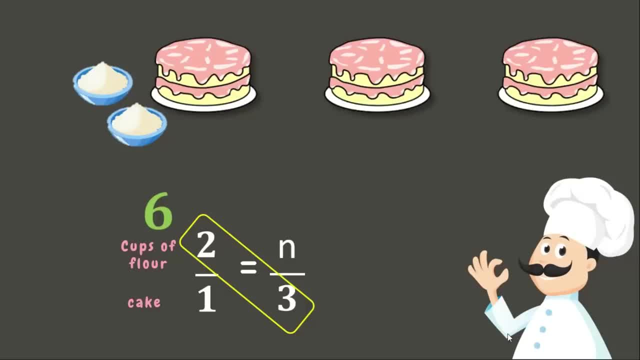 While one times n is one n, But we are only going to write one. The next step is to divide the products. Six divided by one is six. Great job. This means that we need six cups of flour To make three round cakes. 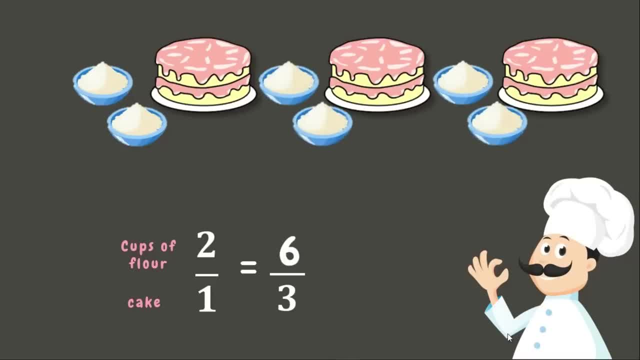 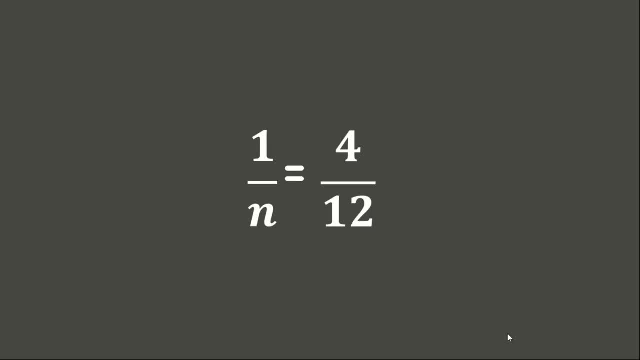 Wonderful. Let's have another example. Let's say we have this proportion. Let's find the missing term. Again, we will use cross multiplication method. Twelve times one is twelve, n times four is four. n Let's only write four. 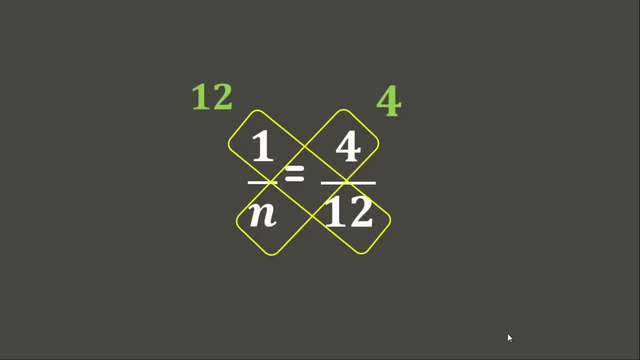 Now let's divide the products. Twelve divided by four is? You are right, It's three. Therefore, the missing term, or n, is equals three. Good job, Now let's try this one. How are we going to find the missing term n? 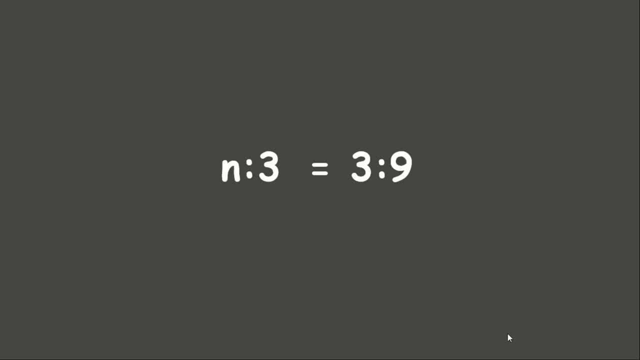 We are going to multiply the means and the extremes. Three times three is nine. Nine times n is nine n, But let's only write nine. Now let's divide the products. Nine divided by nine is one. Therefore n equals one.